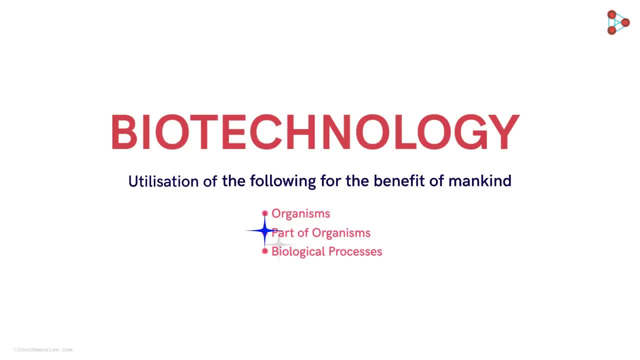 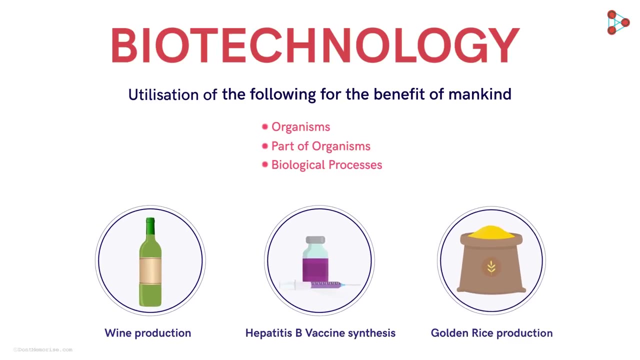 Let's also understand how an organism or a part of it, or some process is produced. We know that the processes can be used to harvest important products for mankind. Let's take examples of wine production, hepatitis B vaccine synthesis and golden rice production. Let's have a look at each individually. 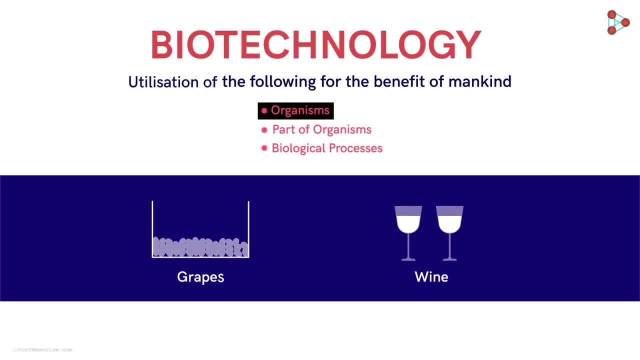 Now, wine is usually made from the grapes. How can grapes, which are fruits, get converted to a beverage like wine? Well, this is where the micro-organism named yeast comes into play. It feeds on the sugars present in the grape juice and releases alcohol and carbon. 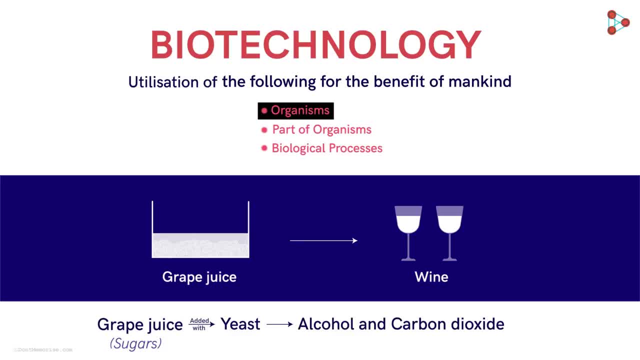 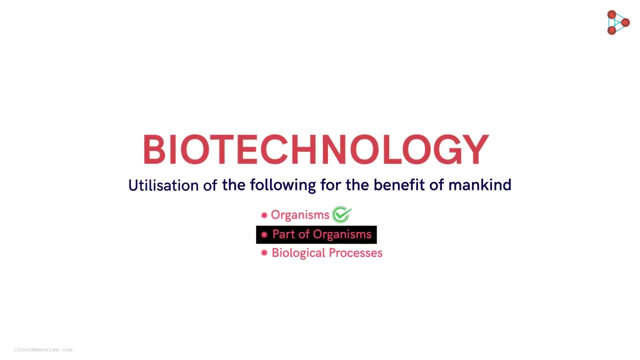 dioxide as by-products. Here a complete organism is used for the processing of grape juice and to convert it into wine. This was the first part of the definition. The second part of the definition states that a part of the organism can be used. So how can that be done For this? let's have a look. 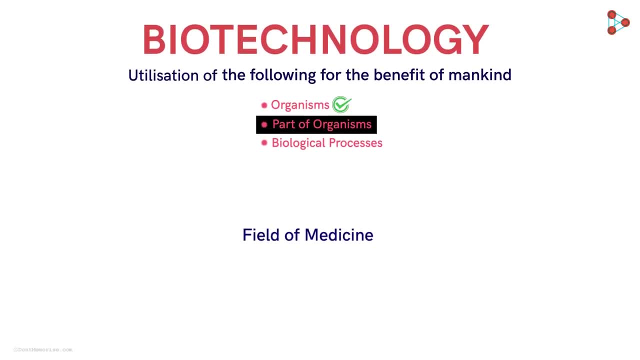 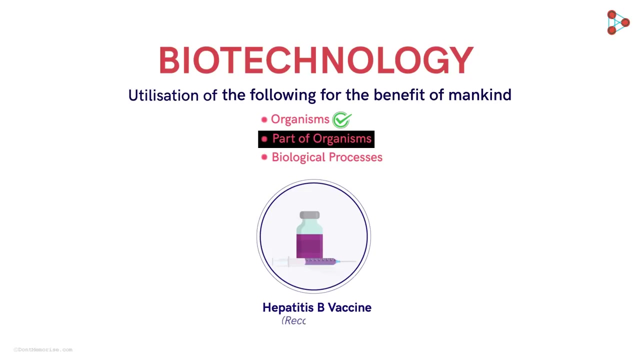 at the application of biotechnology in the field of medicine. Well, the emergence of biotechnology has been nothing less than a boon for the medical industry. Everything ranging from vaccines to gene therapy has raised the standards of healthy living. Now let's take hepatitis B vaccine as an example. This vaccine has a recombinant version. 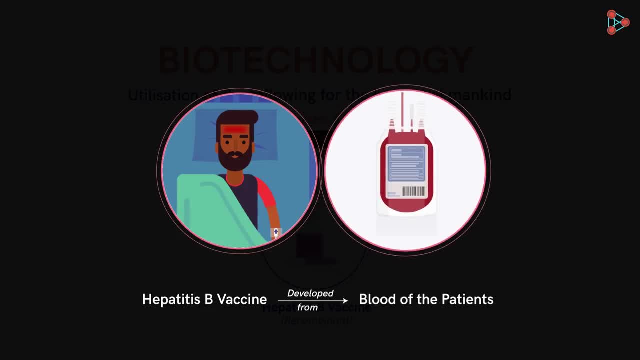 Previously, hepatitis B vaccine was developed from the blood. Now let's take hepatitis B vaccine as an example. This vaccine has a recombinant version. Previously, hepatitis B vaccine was developed from the blood of the humans who were already suffering from hepatitis B, But this was very painful for the patients, as the amount of blood required 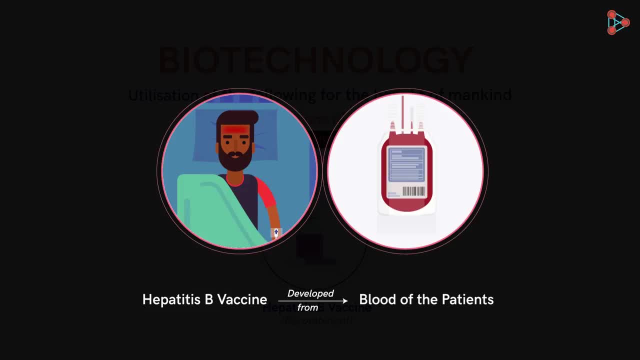 for vaccine production was too high, So extracting some particular amount of blood of the infected person was very excruciating, And as the vaccine was derived directly from the patient's body, there could be negative reactions in the receiving candidate. With the development of biotechnology, new vaccines are being developed in the field. 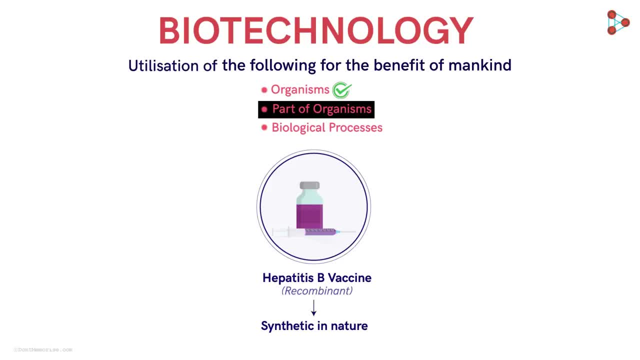 of medicine. The new vaccines that are synthetic in nature started getting produced On the similar lines. the commercially available hepatitis B vaccine is now being synthetically made by utilizing a small part of the pathogenic virus. It's also known as recombinant hepatitis B vaccine. 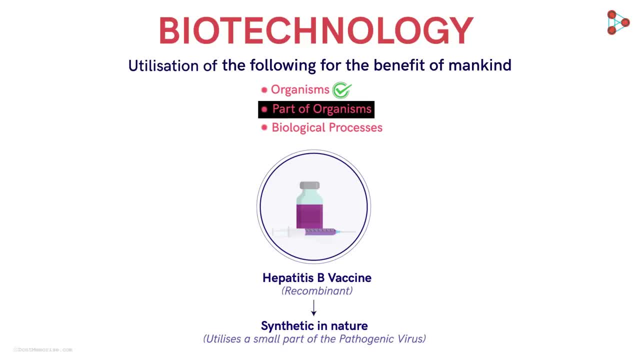 And studies have shown that getting infected with hepatitis B is nearly impossible if a person is injected with recombinant hepatitis B vaccine. So the new vaccines that are being produced are now being made by utilizing a small part of the pathogenic virus. Isn't this a miracle? 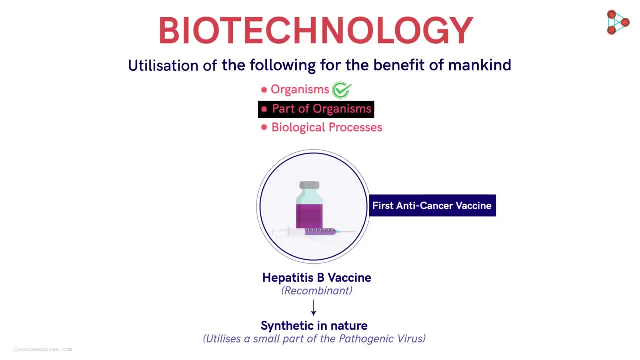 It is equivalent. This is also known as the first anti-cancer vaccine, And why so? Because it's proven that the vaccine helps in reducing the chances of developing liver cancer. This is one example of how, apart from any, organism can be used for product development. 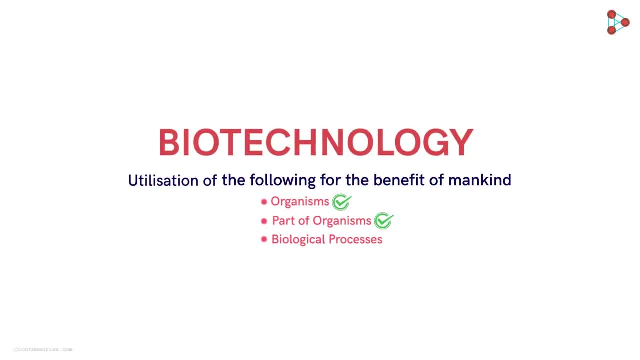 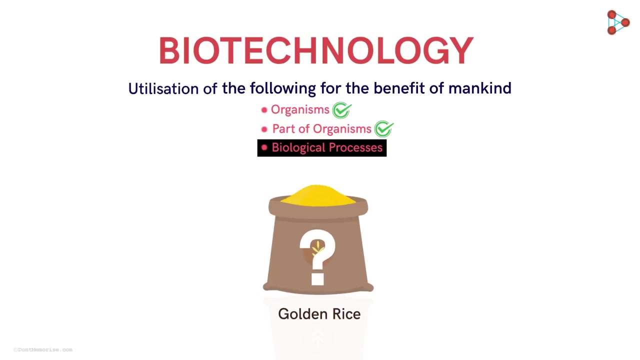 Now that we've glanced at the two examples of application of the biotechnology, let's move ahead to the third one. The last part of the definition stated the use of a process. Let's take the golden rice as our third example Is the rice made of gold. 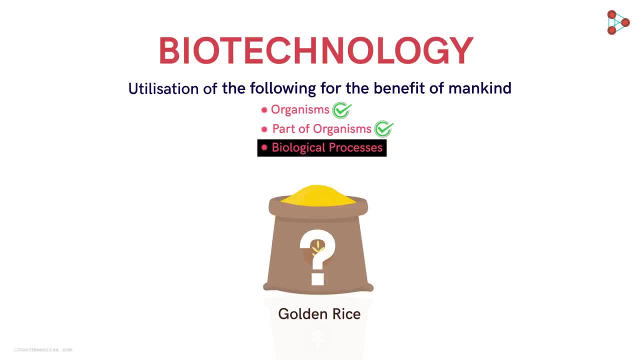 No, absolutely not. Then why is it called golden rice? Well, the rice we usually see is whitish in colour. However, the golden rice we're talking about is a modified version, which is yellowish in colour, Hence the name: golden rice. 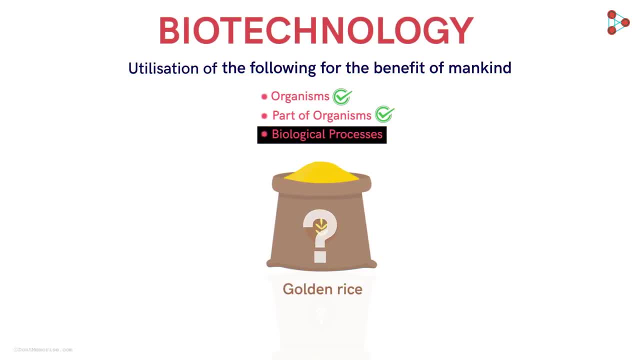 But what makes this rice yellowish and so important? It's the presence of beta-carotene in the rice. And what is that? Beta-carotene is a red-orange coloured pigment which gets converted to vitamin A in the human body. We all know the importance of this vitamin. 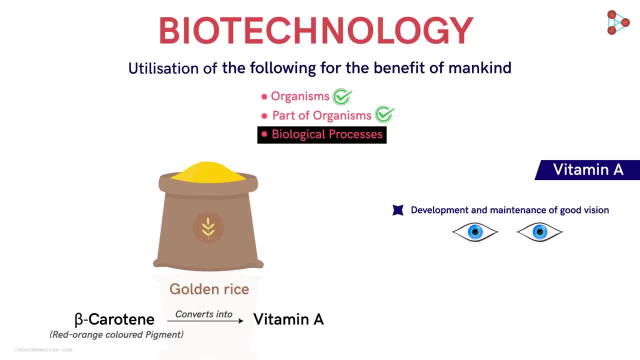 It is most essential for the development and maintenance of good vision. The difference: The deficiency of vitamin A causes vision related issues and malnutrition. Any idea why was only rice chosen for modification? That was because the staple diet for a majority of the population in the areas affected with. 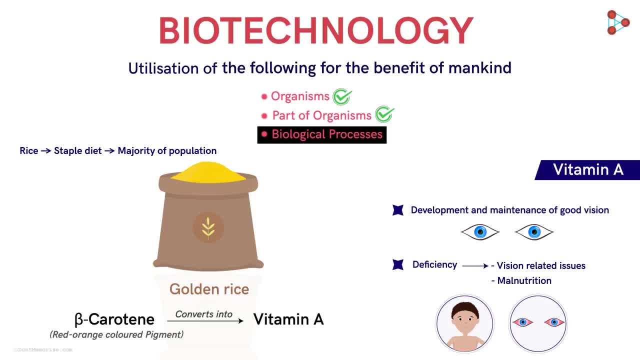 vitamin A deficiency was rice. So to minimise the deficiency, this variety of rice was developed. The modification of rice was done by exploiting a biological process. Now what This is? a process making it a classic example of biotechnological achievements. This variety of rice falls under the category of genetically modified organisms, abbreviated.